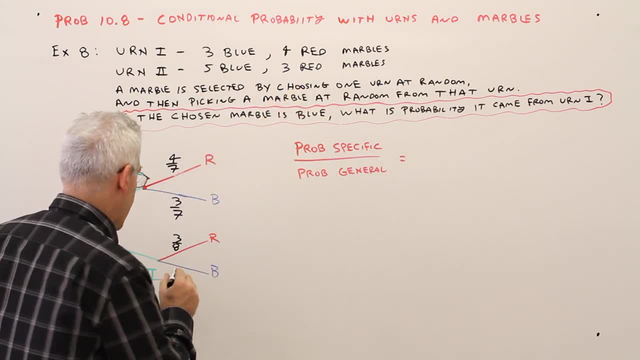 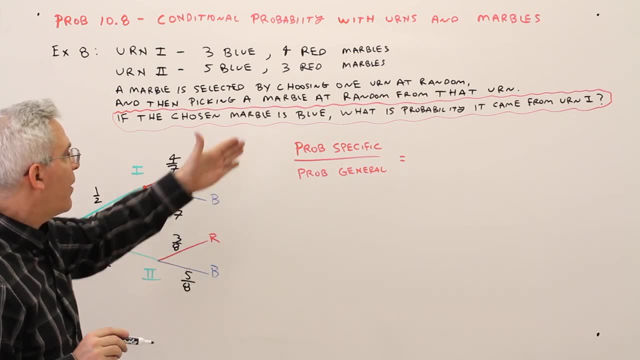 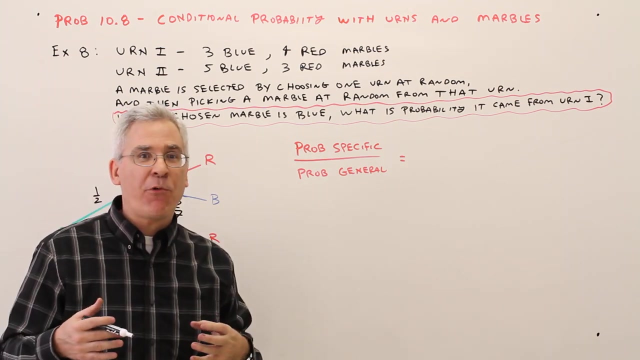 For picking blue 5 out of 8.. Okay, so then, what I'm going to do is I like to do this analysis over here For conditional probability, with these tree diagrams, I think, of the probability of the specific branch over the probability of just the general branches in general. 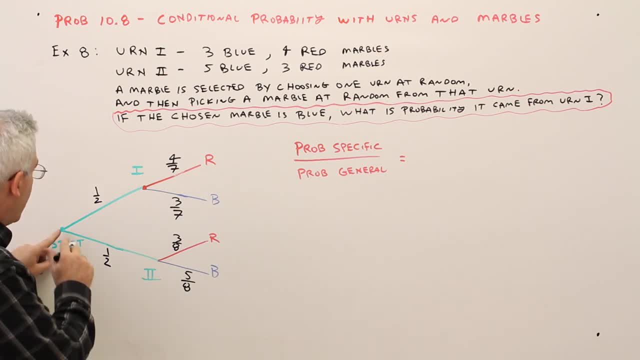 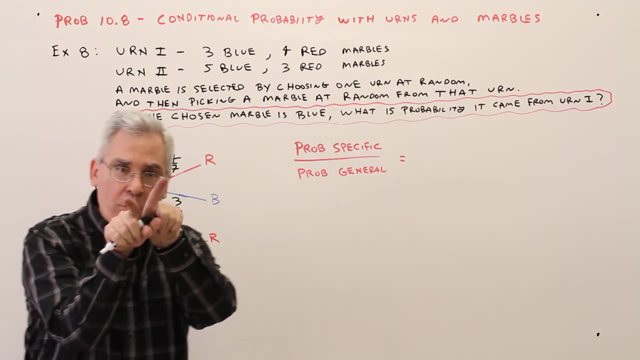 Okay, do note one thing. I've got a starting node here, I've got a half and a half a starting node here, 4 sevenths and 3 sevenths. They add up to 1 from each node. Okay, so 1 there, 1 there and 1 there. 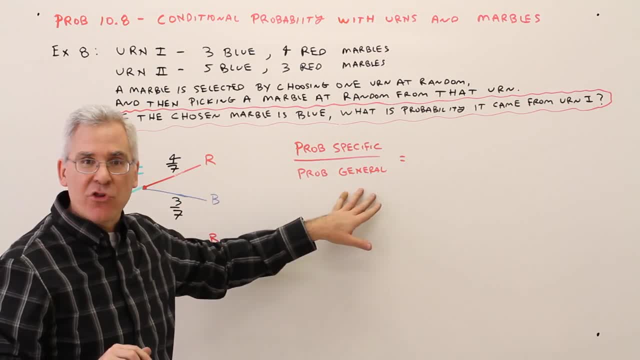 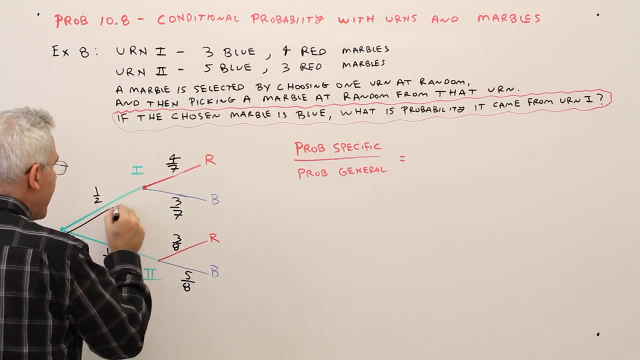 Okay, so let's see, Let's talk about the probability in general. the chosen marble is blue. so, out of all the branches where the marble is blue, So this is a branch where the marble is blue and this is a branch where the marble is blue. 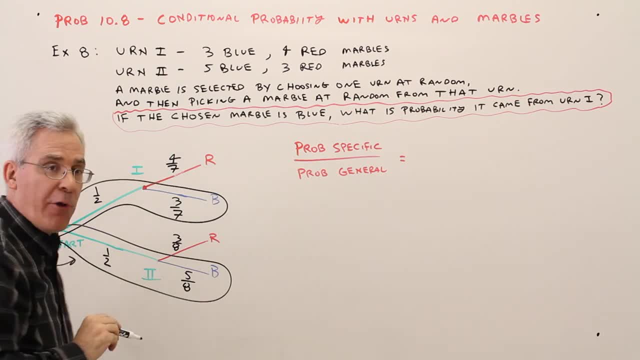 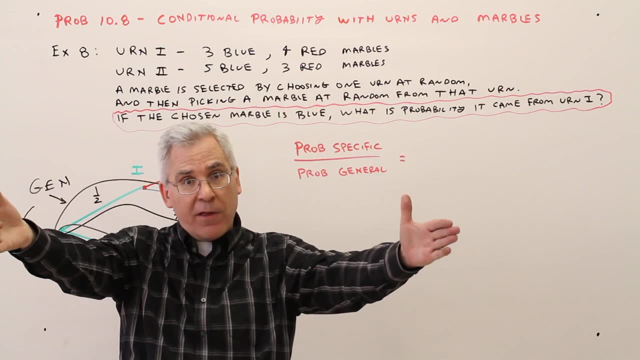 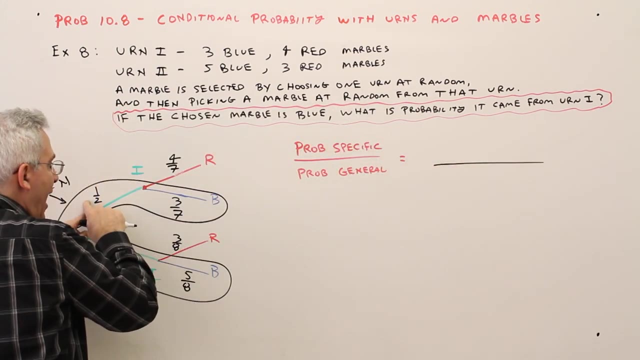 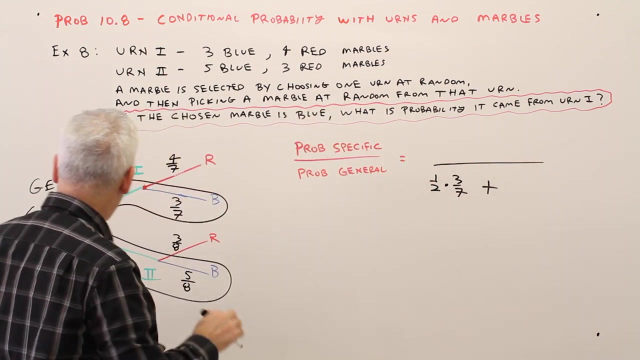 So I'm going to write general for both of those two branches And when I go along a branch I multiply and if I've got this branch or this branch I add. Okay, so for my probability in general it's going to be 1 half times 3 sevenths or plus. 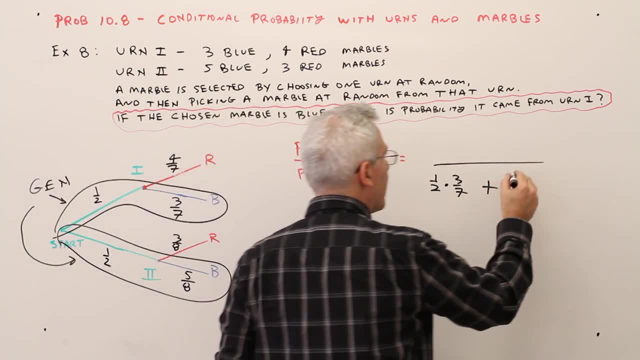 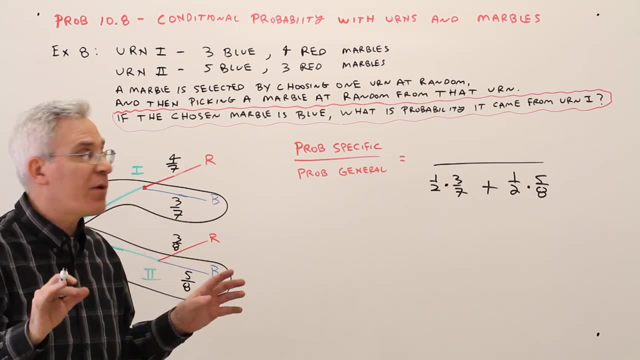 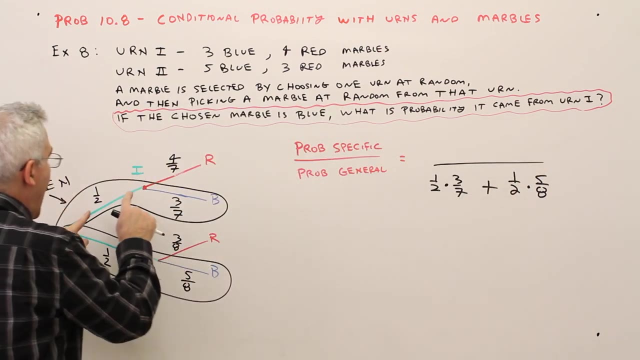 1 half times 5 eighths. Okay, so that's all of my general scenarios. Now my specific. I want to be blue and earn 1.. So, blue and earn 1. And earn 1, this one right here is my specific branch. 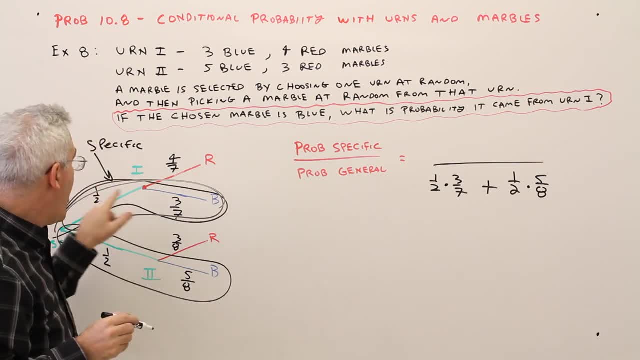 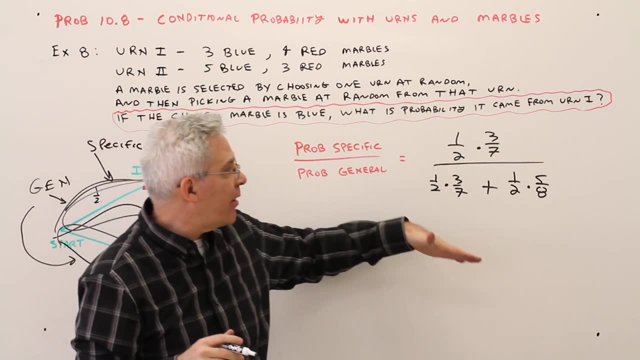 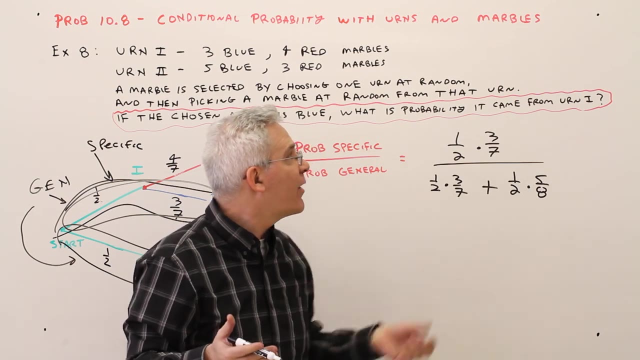 Just that branch. So probability of specific 1 half times 3 sevenths. And then just be careful with your calculator. You could use the numerator denominator key. You do have some repetition here if you want to use that. And if you calculate this, you get 24 over 59.. 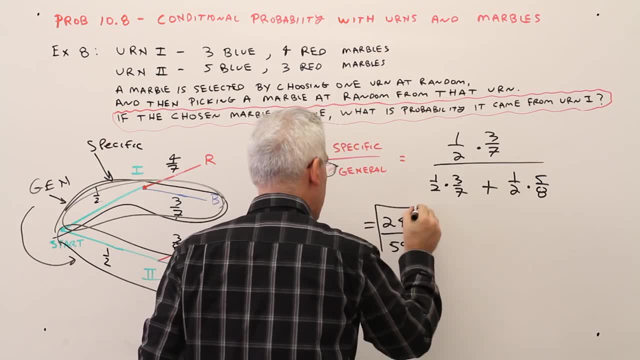 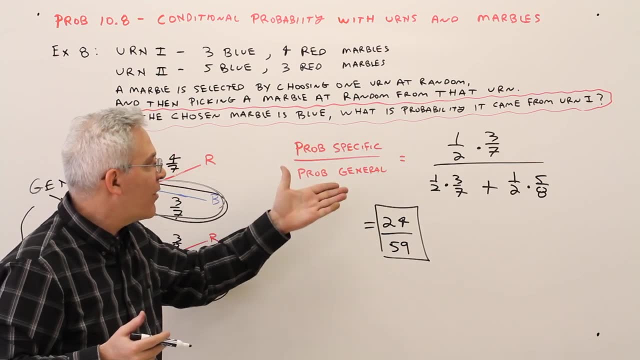